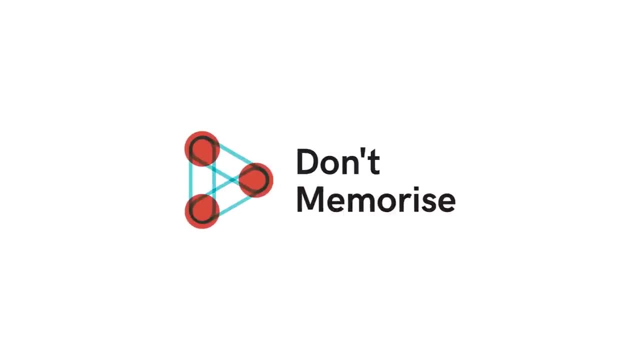 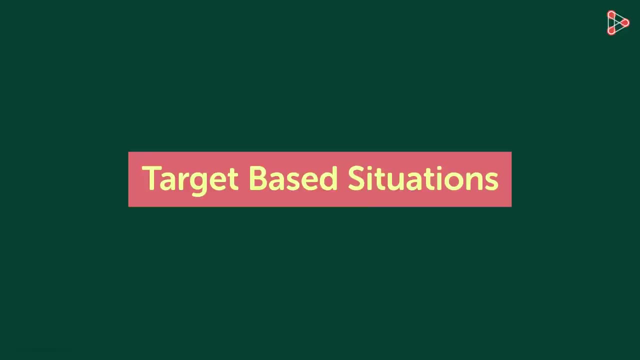 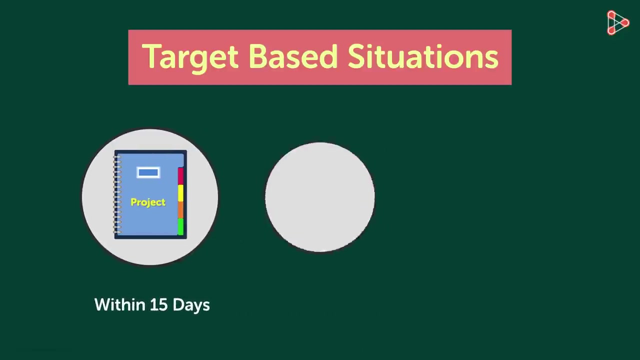 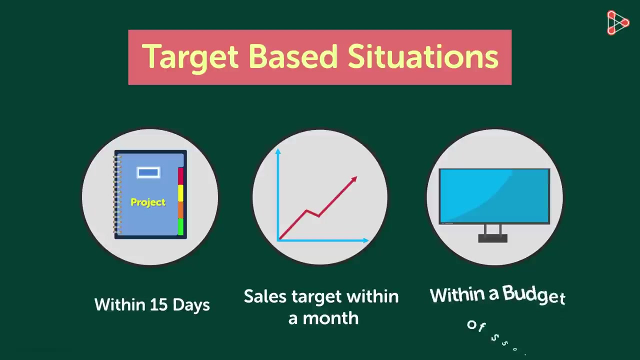 We all come across many target-based situations in our day-to-day life. Can you think of any? Say: a student has to complete a project in 15 days. Or a salesperson has to achieve a sales target within a month. Another person has to buy an electronic gadget within a budget of $500.. 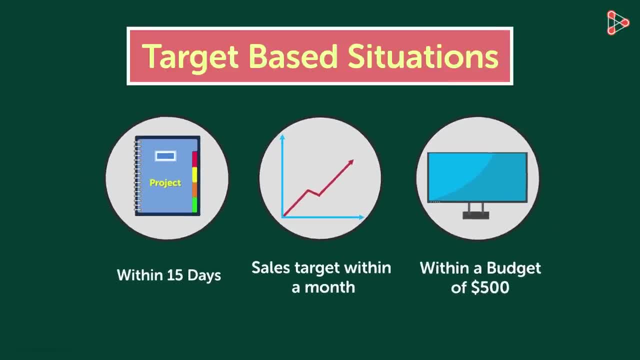 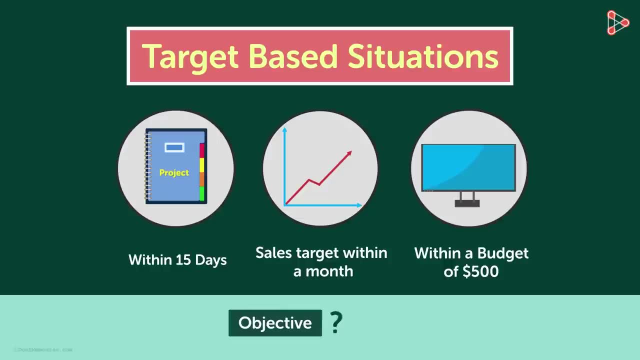 Go through these situations and try to find out the main object to be achieved by each person individually. What is the objective of the student in this case? Yes, she wants to achieve the maximum score in this project. Can you tell me the objective of a salesperson in this case? 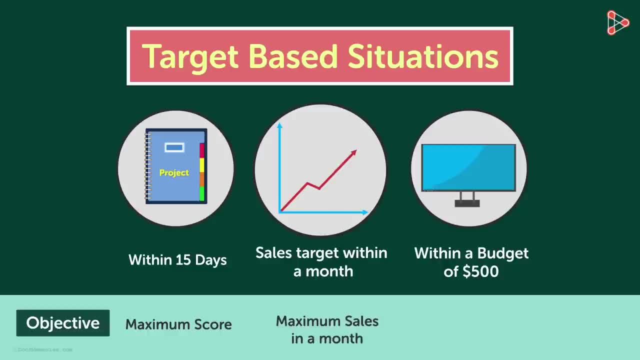 Yes, he would aim to achieve maximum possible sales in a month. What do you think would be the objective of a salesperson in this case? What would be the objective of the person buying a gadget? She would try to minimize the cost as much as possible. 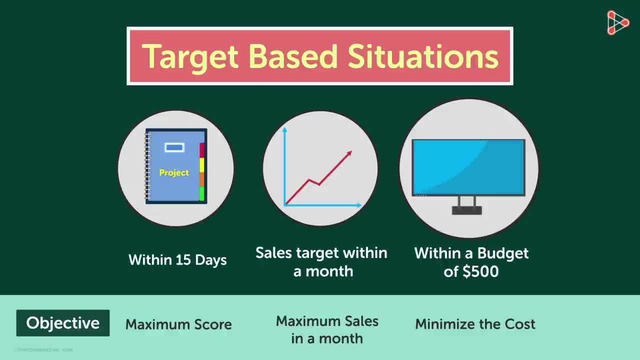 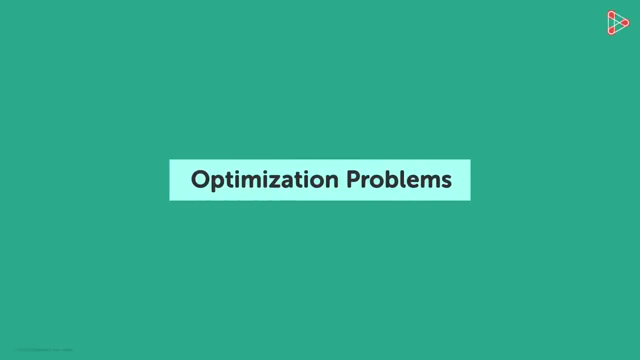 She'd buy a gadget that falls within her budget. We can see that in each of the cases above, the objective of the situation was to maximize the benefits or minimize the cost. Such types of problems are called as optimization problems in mathematics. Thus, an optimization problem may involve finding: 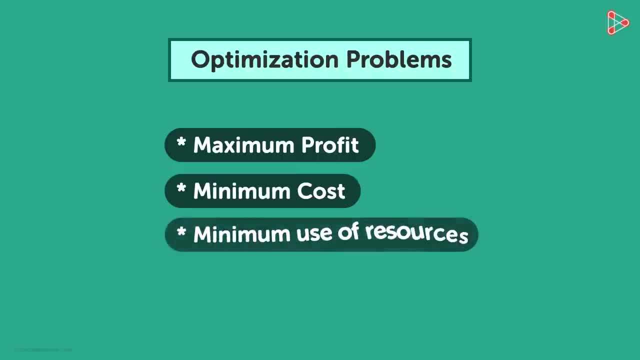 maximum profit, minimum cost or maybe minimum use of resources. There can be many more examples from our day-to-day life which need to be solved using the optimization technique. The problems can be as simple, as stated above, but could get complex depending on the situation. 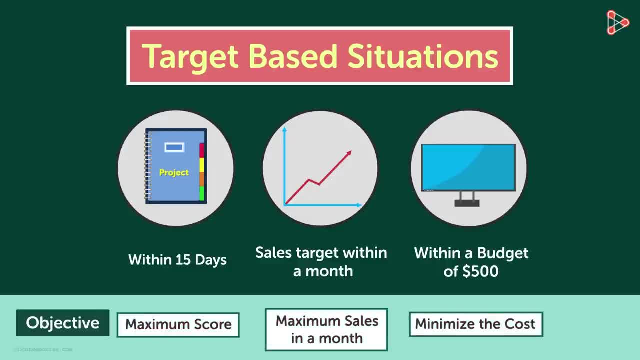 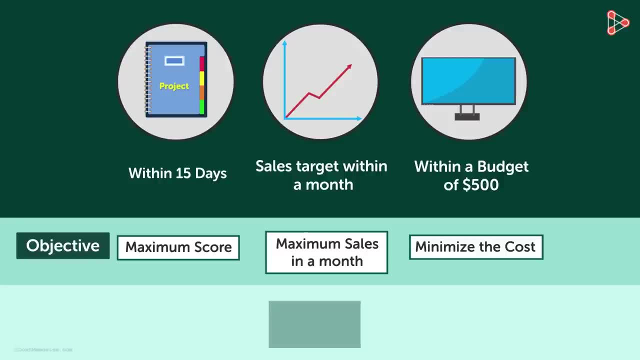 We have already discussed about the objectives of the three given situations. Now we will look at the other important factors. We will identify the limiting factors in each case. What does that mean? Well, in each case, there is a scarcity of some resource. 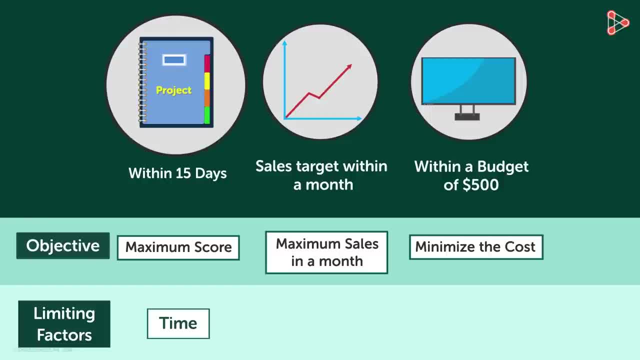 Like in the first case, the time limit to complete the project is limited. Time to be allotted for completing the project is limited to 15 days only. Likewise, in this case too, time is the limiting factor. The salesperson has to sell the maximum possible.